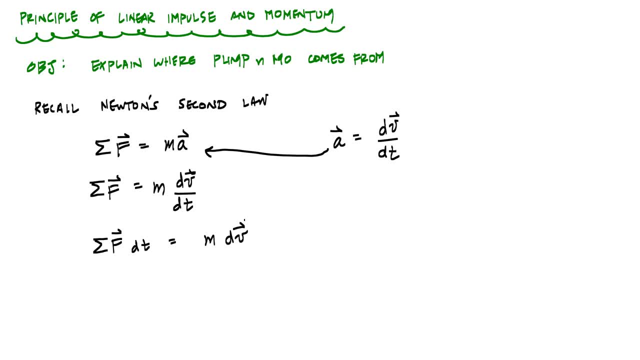 I have here is, and set up now, that I can integrate with respect to time on the left and with respect to velocity on the right, like that. yes, and when I go ahead and I rearrange or I evaluate this some more, I know that this right here and 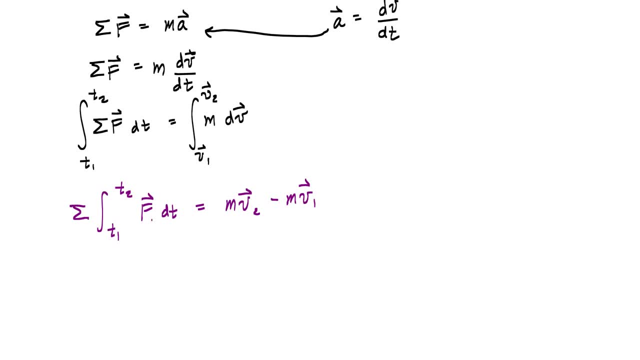 what I have here is this force and times times time on the left, and this force, times time, which has units of like Newton seconds or pounds seconds. is it an impulse? it's like a punch. this is the sum of all the impulses. and on the right, 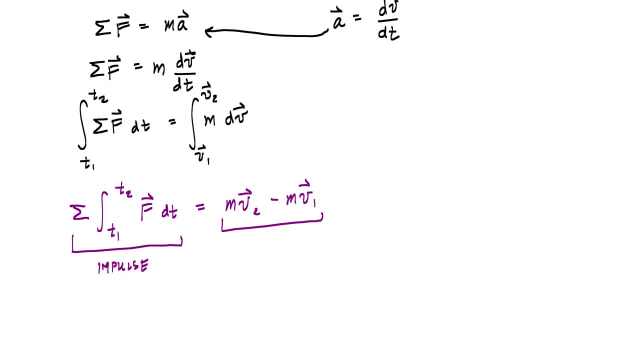 right here. this mass times velocity, you probably remember, is momentum, and so this is a change right here: change in momentum and what this? what this relationship says is that the sum of all the linear impulses on the particle is equal to the change in momentum. I could even rewrite this another way, as 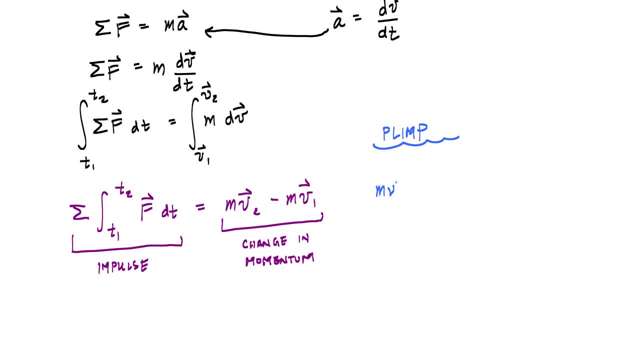 you can see in this example, I'm going to go ahead and I'm going to go ahead, and, and I'm going to go ahead and I'm going to go ahead and I'm going to go ahead, and the principle of linear impulse and momentum, and if I take this MV1 plus the 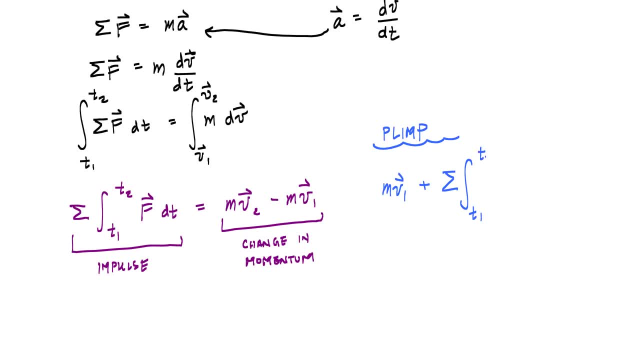 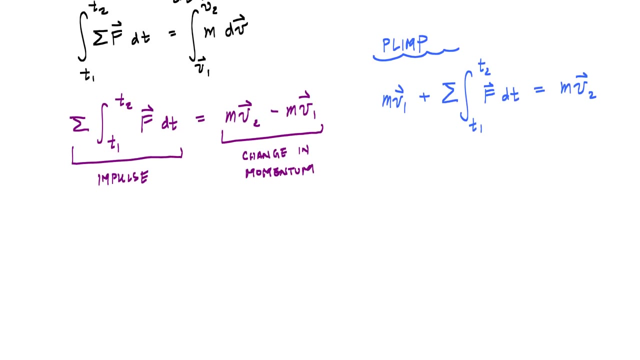 sum of all the impulses from t1 to t2 is equal to MV2. like this right here and notice: these are all vector quantities. this is something that we can break up into two equations or three equations, depending on how many dimensions that we're working on, but if it's 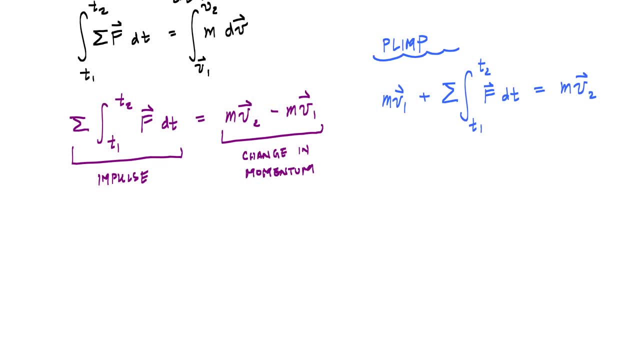 two dimensions. that means you can break it up into like a horizontal and vertical component. the thing i like to do is make sure that we have a schematic here, and so what we have is like a particle that is moving with one, a specific type of momentum: m v, one like this. so you know someone. 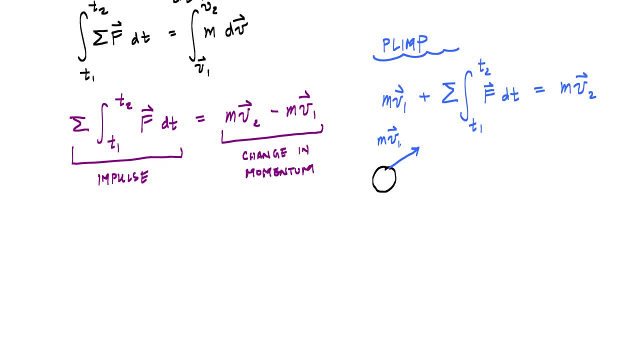 is running in one direction or driving in one direction, and then it gets impacted or punched. the particle gets punched by all these forces that are acting on the particle for a certain period of time. you know there might be a force here, boom. that's applied for a certain period of. 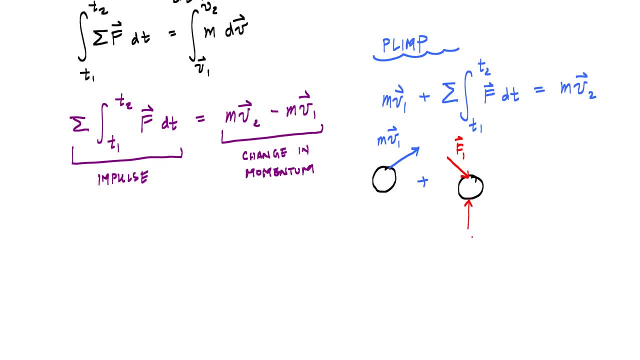 time or that same period of time. we have a force here applied for a certain period of time, like this: okay, and each of these over that time can be turned into an impulse, t1 to t2, that's acting on the particle t1 to t2 like this and whatever resulting impulse, that is, that comes out to a certain stage of. 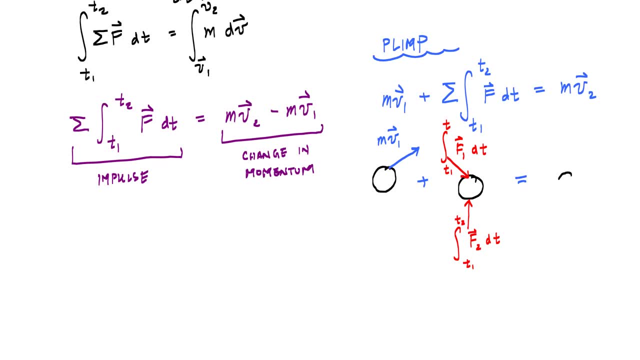 momentum, it changes, let's say, the direction and the velocity of the momentum of the particle to a different direction. MV2 like this, yes, so this schematic. right here I'd like to emphasize drawing three parts to the schematic. when drawing problems with the principle of linear impulse and momentum and- and I think that's a good habit- 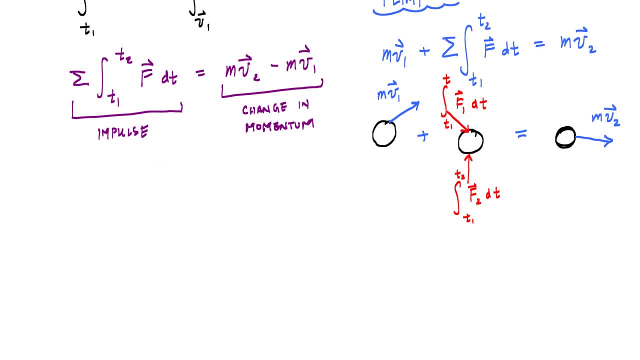 to develop. all right. so, as you can imagine, the linear impulse, or this impulse term right here is, is some sort of integral, and so that integral could actually, you know it, basically, you could be given force as a function of time, like this, and whatever the shape of the curve is, you know it. 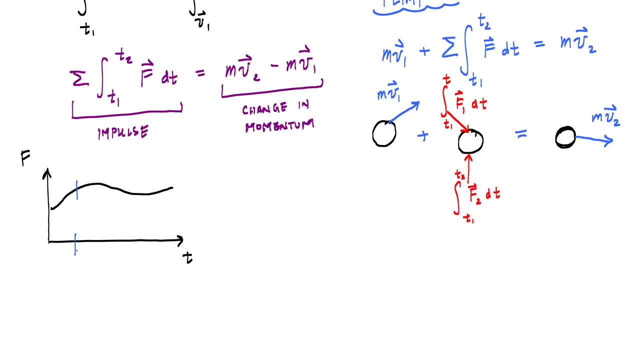 could be doing this and If we're interested in the impulse from, let's say, T1 to T2, right here, basically this area, the magnitude of the impulse would represent the area under the curve right here: T1 to T2, F of T, DT. 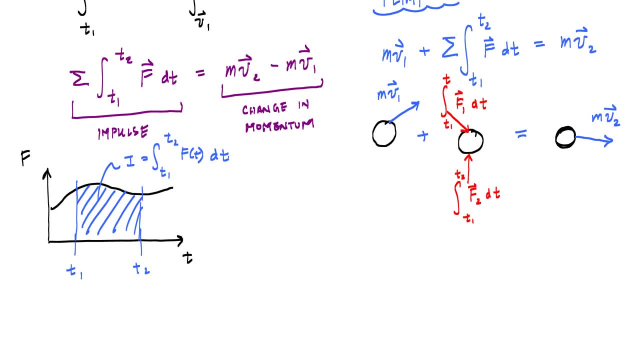 And whether it's constant, linear, parabolic, cubic, whatever sinusoidal, you can integrate that. It's just math And so that's how you would calculate the impulse, And usually you know, like if you have a motor that's driving or like pulling on a cart. 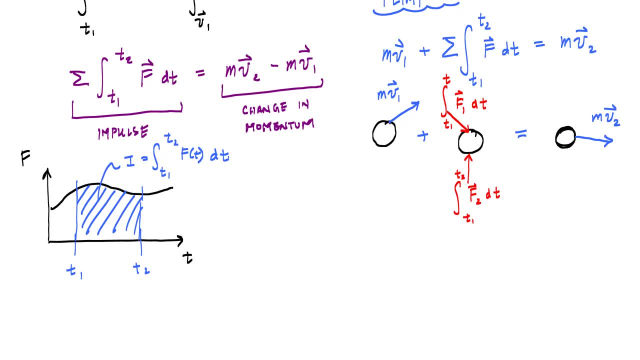 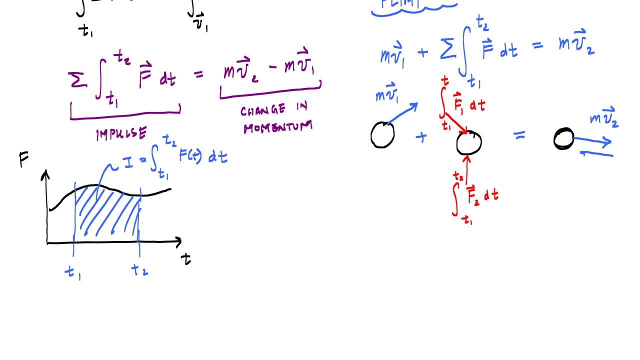 that will have, you know, a time-varying force on the particle. The other thing I want to just remind you is that here this is a vector equation, And so that does mean that we can break up this principle of linear impulse and momentum into scalar equations.